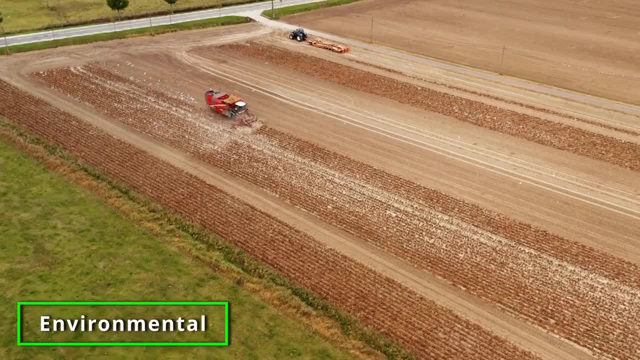 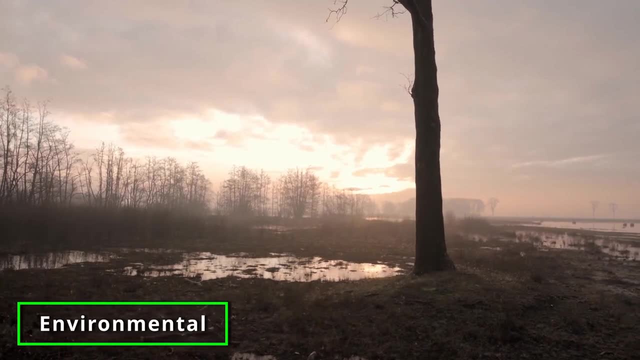 Careers in soil science may be of interest to you if you want to work with soil and water quality, agriculture, wetlands, or conservation. Careers in this field often involve working in laboratories and doing fieldwork, but may involve some office work as well. Quite frequently, 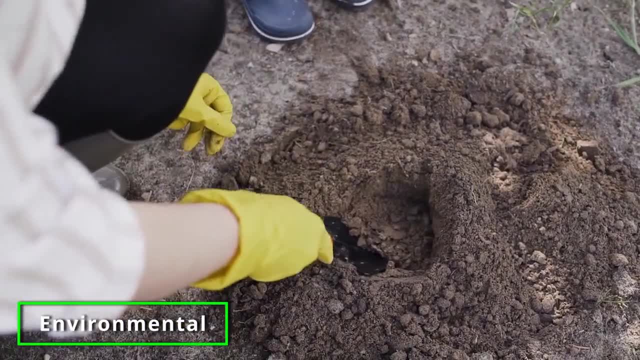 soil science careers may also be found in the natural resources field. Median pay for soil scientists is $74,000 per year, which is about $100,000 per year. Soil science careers may be of interest to you if you want to work with soil and water quality, agriculture, wetlands, or conservation. 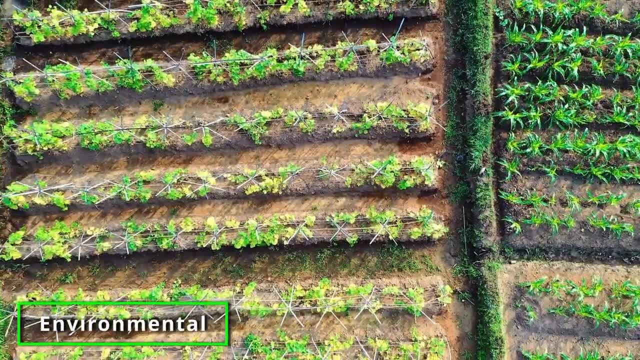 Typical entry-level careers require a bachelor's degree, and careers in this field are projected to grow by 9% by 2030, which is about average. 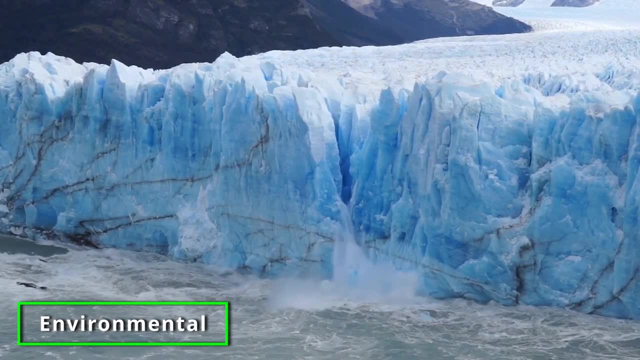 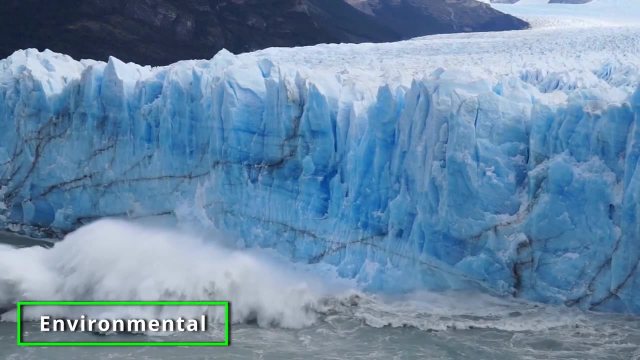 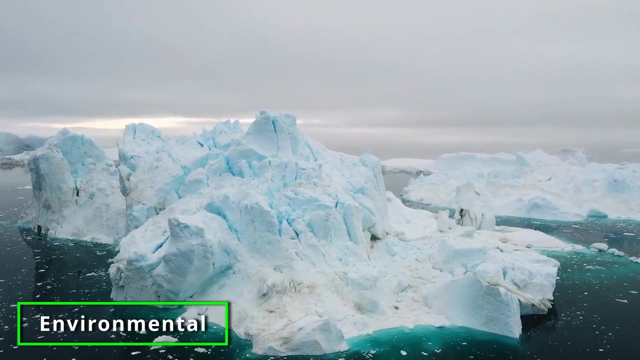 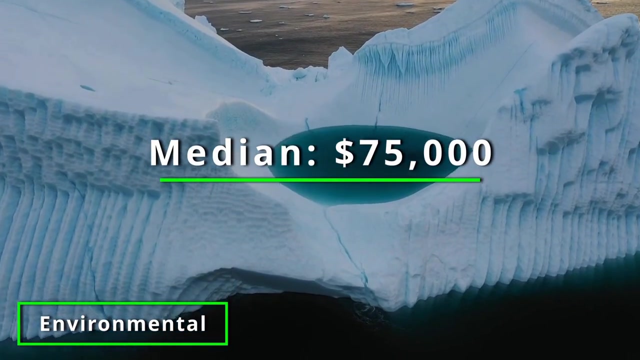 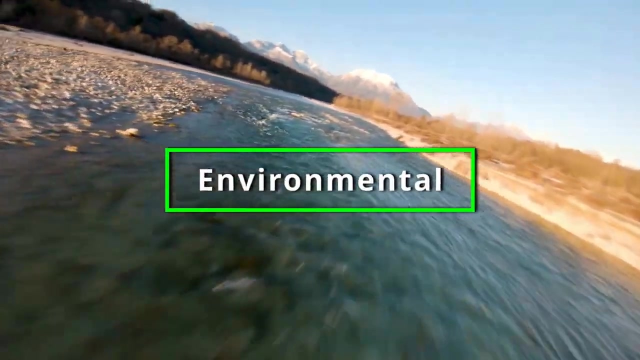 Glacial geology is the study of the physical properties and movement of ice sheets and glaciers. A glaciologist's goal is to find out whether ice sheets are growing or shrinking to learn about global sea level and climate changes. The education required is generally a bachelor's degree in geology. However, employment as a field researcher, research requires a master's or doctoral degree in glaciology. The average yearly income is $75,000, and the jobs are increasing at 8%. Environmental careers often have overlap with 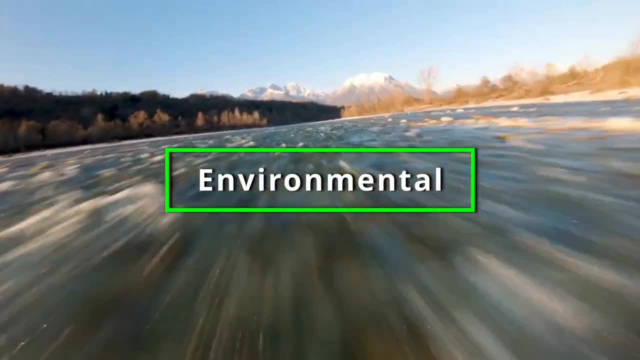 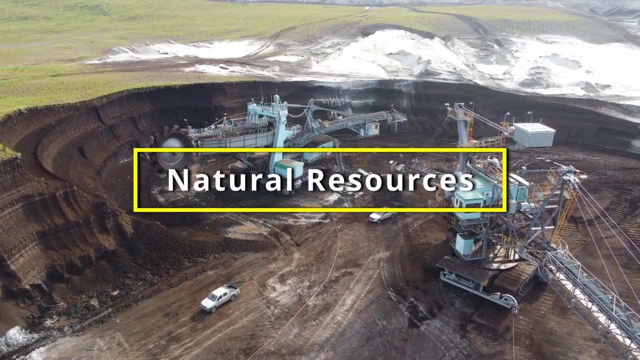 careers in all of the other fields. Many jobs that are typical of what we think of as geology often fall into this field and may involve working for government or in the private sector. The goal of jobs under the natural resources branch is to explore, monitor, and extract natural resources we use to keep society afloat. This includes mining, mining, and mining. The goal of jobs under the natural resources branch is to explore, monitor, and extract natural resources we use to keep society afloat. This includes mining, mining, and mining. The The goal of jobs under the natural resources branch is to explore, monitor, and extract natural resources we use to keep society afloat. This includes mining, mining, and mining. 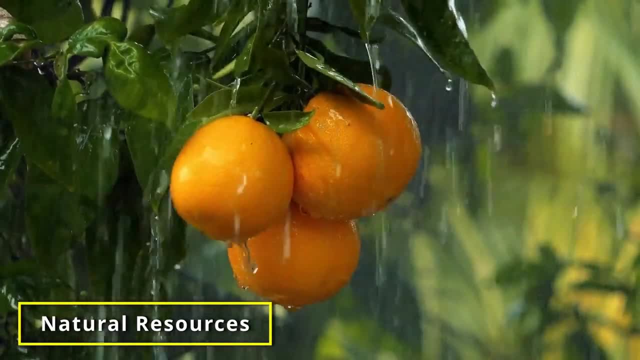 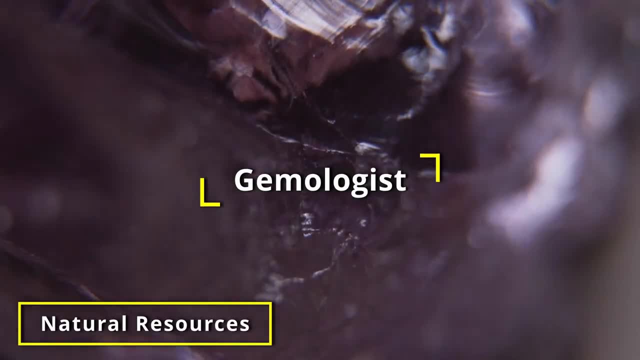 Gemology is becoming a gemologist. Gemstones and other crystals are an important part of industry, technology, fashion, and even the medical sector. As a gemologist, 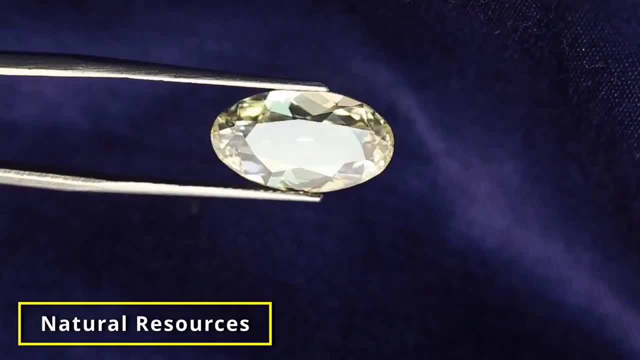 you can analyze both raw and refined samples to determine their type, quality, and value. 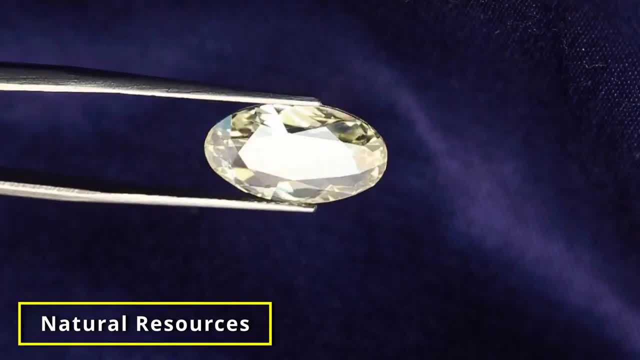 These jobs can be found in both the field and lab. Most time is devoted to the latter for easy access to their hyper accurate instruments including microscopes, calipers, reflectometers, 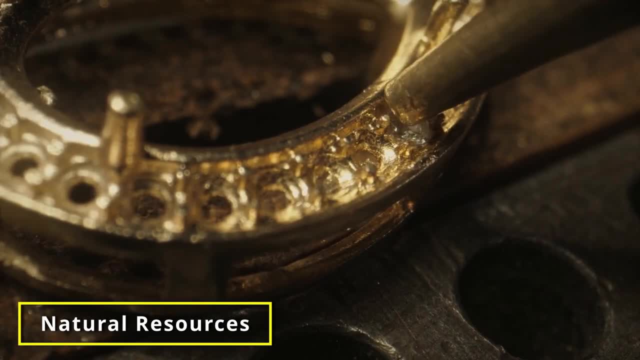 and spectroscopes. Because of the wide range of uses for gemstones, there is plenty of room for interdisciplinary cooperation and engineering. 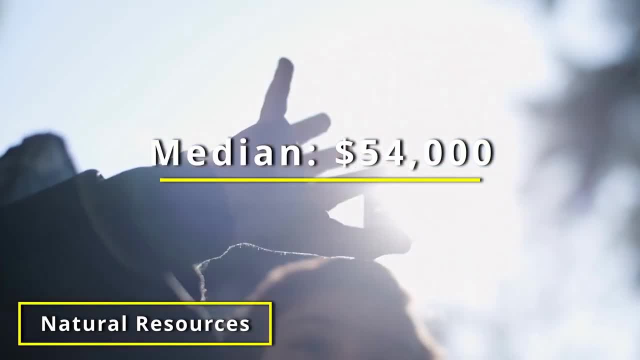 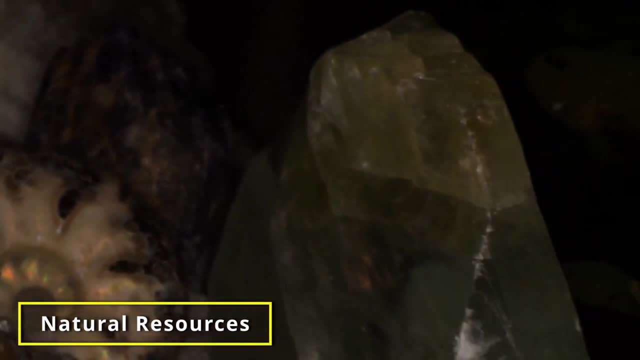 Colleges generally make around $54,000 per year. Getting started in this field may only require obtaining a certification through some trade classes, but for those looking to take their career further, there are both undergrad and graduate level courses at many colleges and universities. 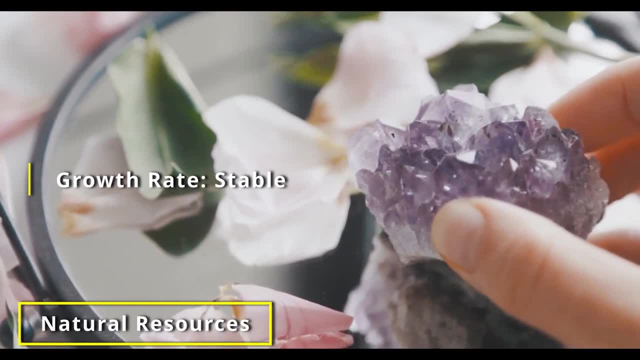 This is a relatively stable pathway expected to not see much change in job availability over the next decade. 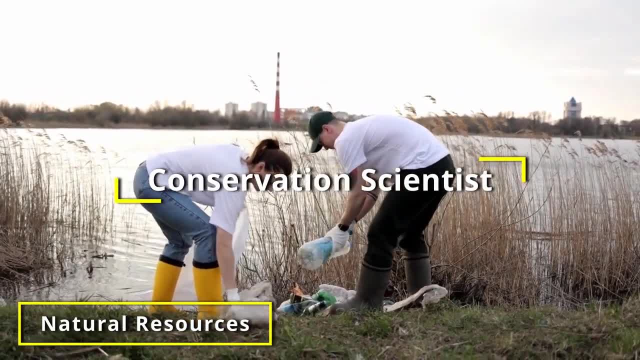 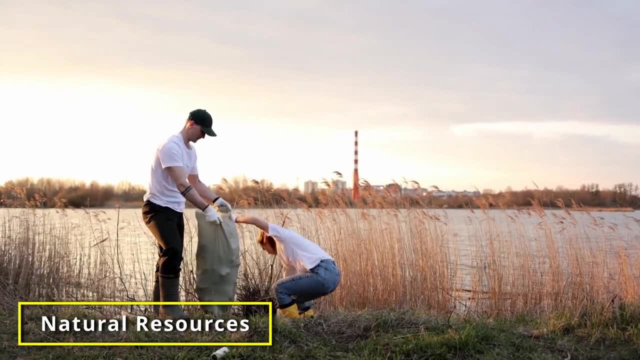 Environmental protection careers can involve monitoring the environment and determining sources of contamination, as well as protecting and managing quality of natural resources, ranging from parks, beaches, wetlands, forests, and other natural resources. 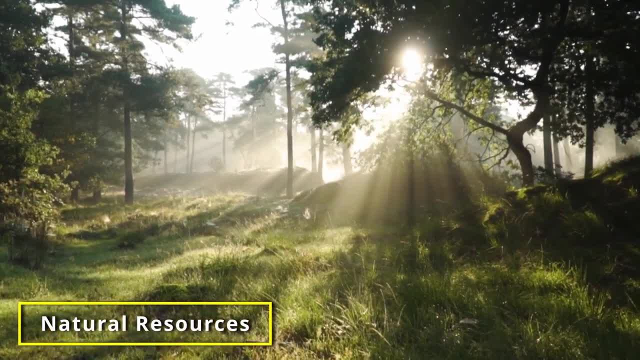 If you are interested in environmental protection and conservation, careers in this field may be appealing. 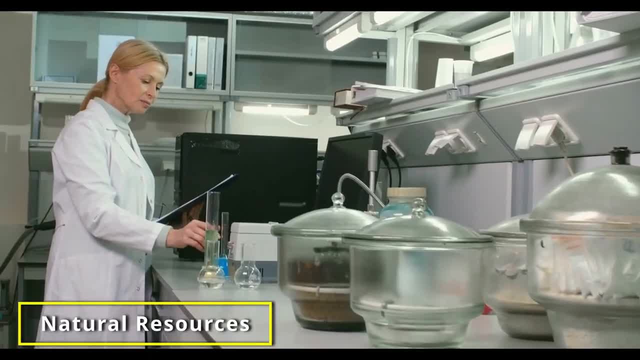 These types of careers often involve office or laboratory work, but may include some field work depending on the level of the position hired and for. 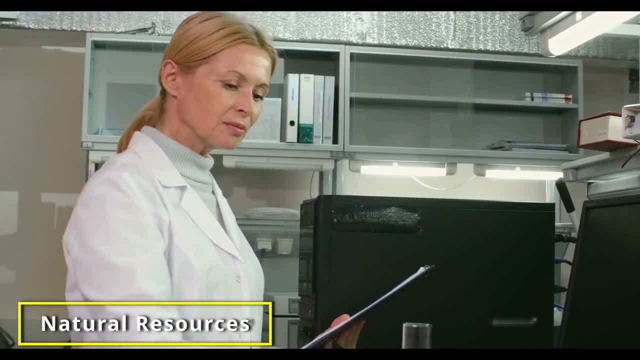 Similar jobs may also be found in both the environmental and engineering fields. Median pay for conservation scientists is $64,000 per year, and typical entry-level jobs require a bachelor's degree. 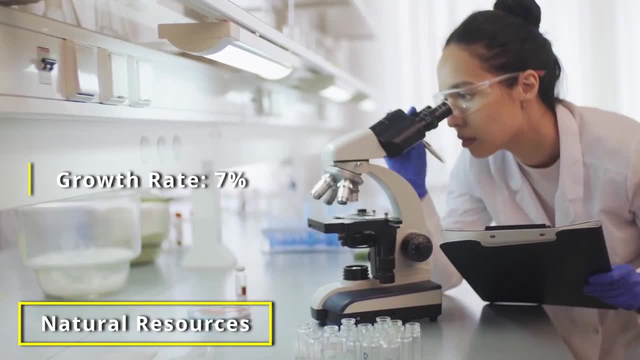 Careers in this field are projected to grow by 7% by 2030, which is about average. 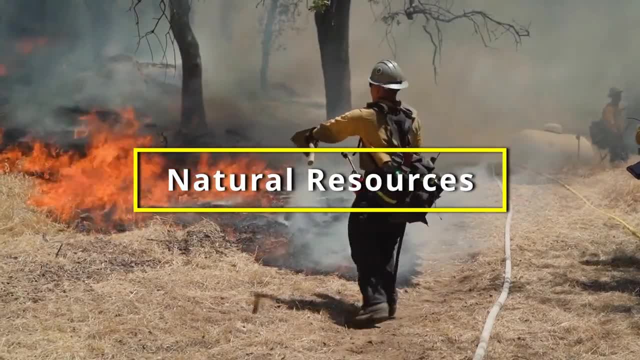 Again, this is just a brief overview of some of the cool jobs to be found within the natural resources sector. Like all the others, they couldn't properly function without the support of all the other branches in one way or another. 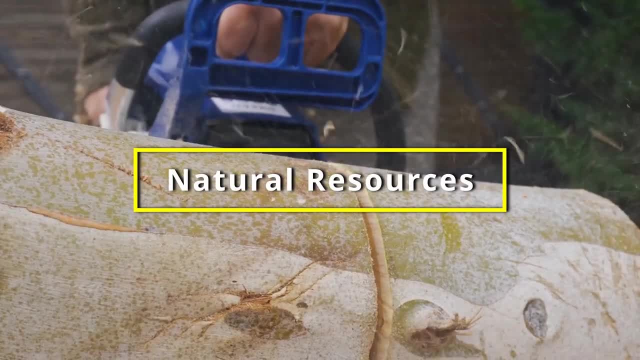 Students interested in natural resources have a great opportunity to help utilize and conserve the resources that are vital to us and the many ecosystems that depend on them. 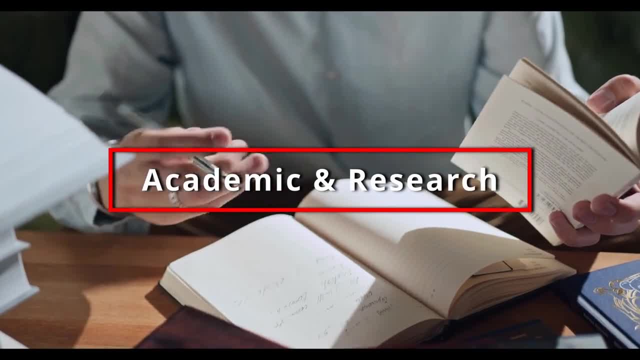 There are also jobs in the academic and research fields as well, most of which require a master's degree or greater to fulfill the tasks and responsibilities of the job. 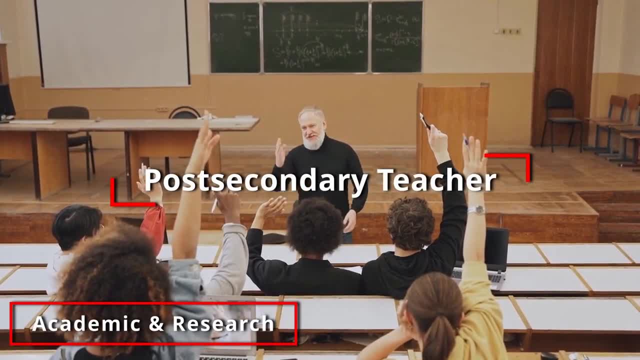 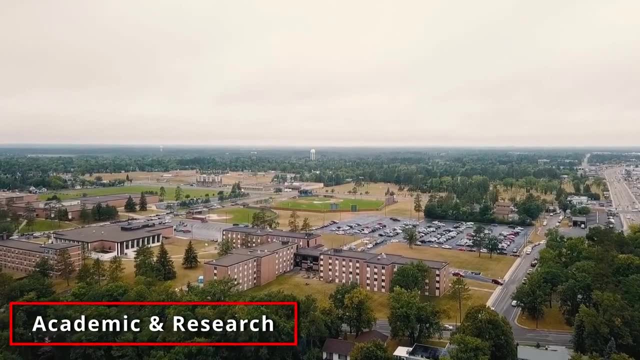 Career focus in post-secondary education varies depending on what classes are available to teach. Typically, professors will be teaching classes similar to the field that they focused on in graduate school, but may be asked to teach entry-level courses. 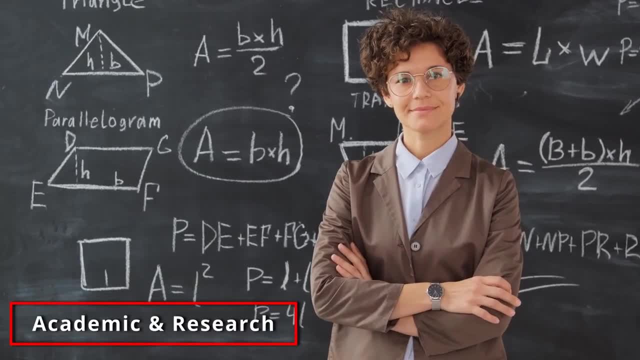 Work environments are typically at public or private colleges and universities, and jobs can be part-time if hired as an adjunct, but many of these positions are full-time. 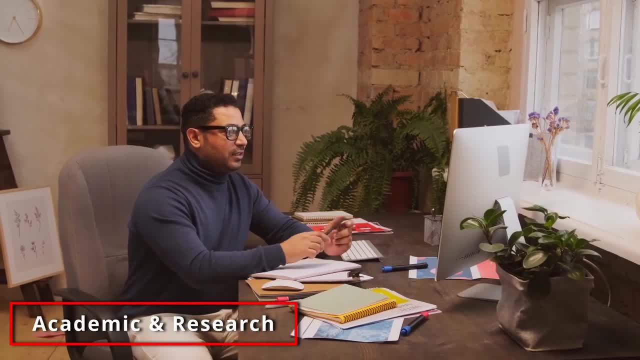 Many post-secondary educators may also have overlapping work in environmental, social, and environmental, natural resources, remote sensing, and engineering fields. 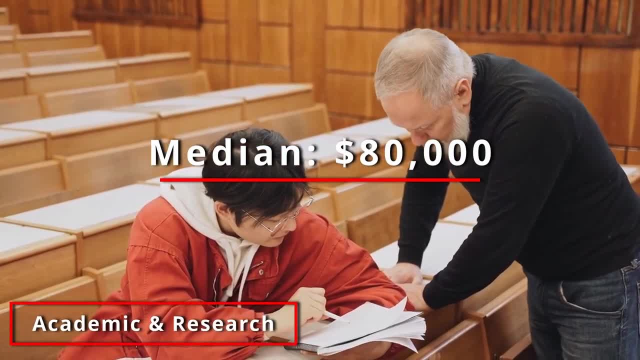 Median pay for post-secondary teaching is $80,000 per year. Typical entry-level jobs require a master's for two-year colleges or a Ph.D. for four-year universities. 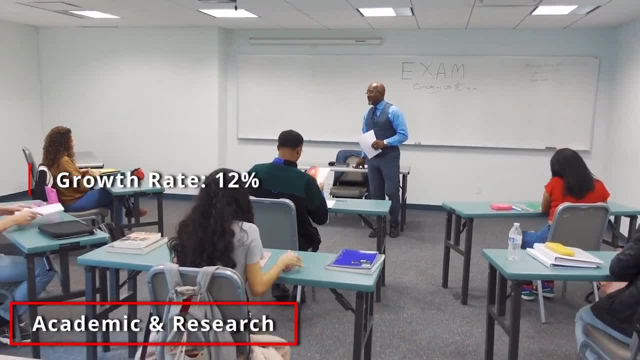 Careers in this field are expected to grow by 12% by 2030, which is above average. There are even geosciences jobs that are out of this world. 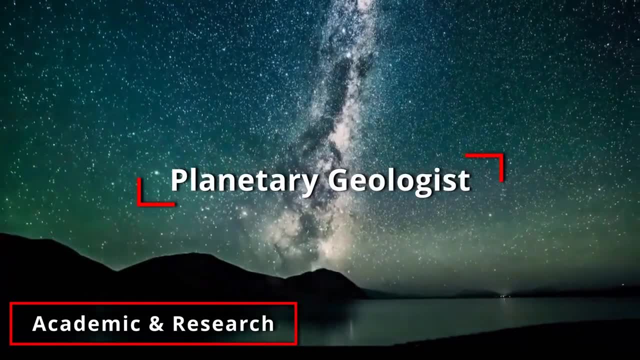 A planetary geologist is someone who studies how other planets and the moons and the asteroids and comets and whatever else is flowing. 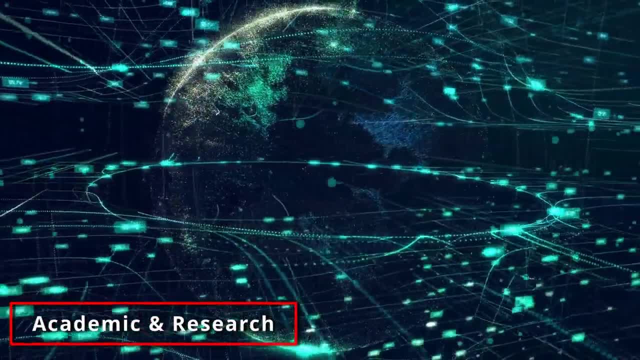 We use what we have learned about how the Earth works to try to understand how planetary bodies work. 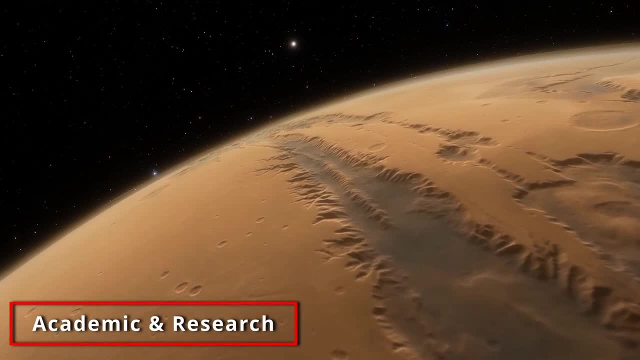 Planetary geologists may focus on mapping out the topography of a planet, extrapolating information from asteroid core samples, or even operate the movements of a robotic exploration mission. 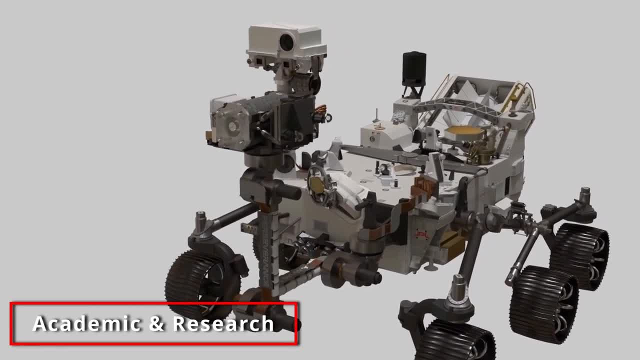 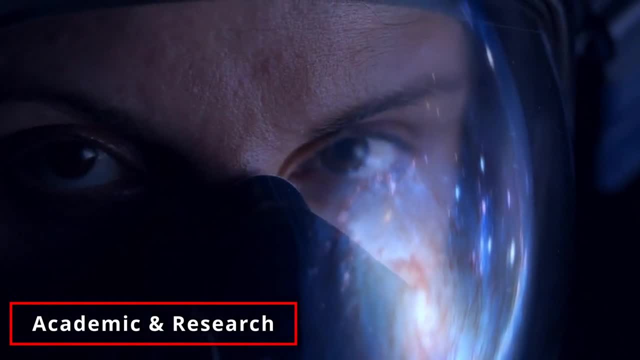 NASA's Marv Rovers have provided an amazing example of planetary geology in action, with scientists working to investigate the surface of that planet for notable geophysical evidence, especially scientists. Science of life. 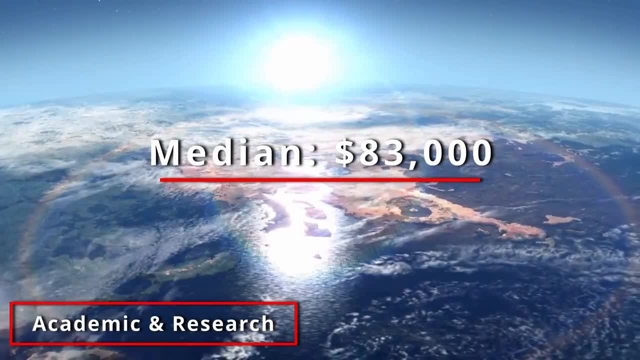 The median income for this job is $83,000 per year, and there is a job growth of 7%. 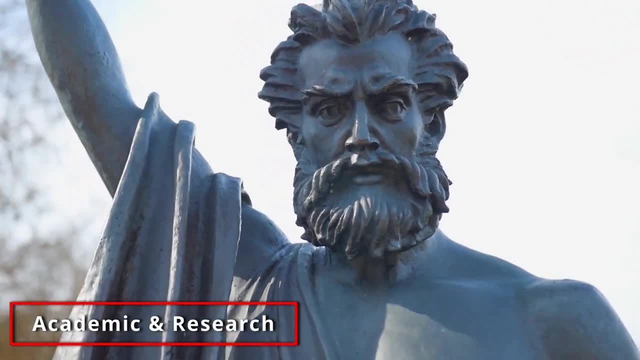 History comes in all shapes and forms, from the philosophers of ancient Greece to the development of supersonic jets. 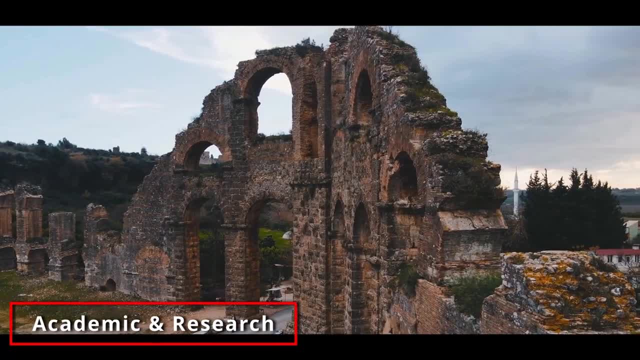 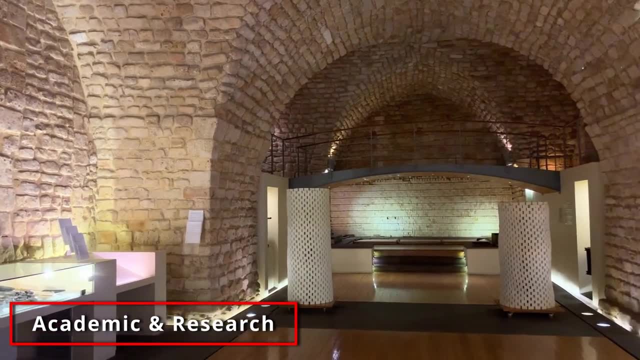 Geology and environmental science students can help preserve history and cultivate curiosity by becoming a natural history or natural science museum curator. Many organizations assign their curators a variety of different duties, but in many cases, this job entails a lot of work. The most important job is acquiring and authenticating specimens. This includes securing funds, overseeing proper transportation, and making sure the subsequent preservation protocols are in effect. With that done, many curators design and monitor exhibits for the museum to make sure events are well coordinated and guests are happy. This job is a great opportunity to preserve the past wonders of the world while educating upcoming generations about how great it is. The median salary for people in these positions is about $50,000 per year. Getting a job as a museum curator or museum curator is a great opportunity to get the experience you need. As a museum curator, I have a goal to achieve. I am a museum curator and I have a mission to do. In addition to the importance of the museum, I am a museum curator and I am an exhibit curator. I am an exhibit curator. I am a museum curator. happy. 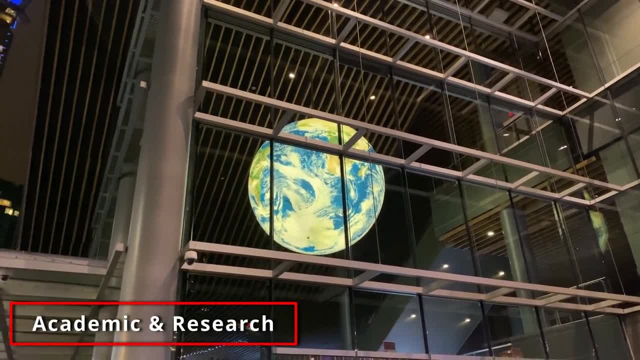 This job is a great opportunity to preserve the past wonders of the world while educating upcoming generations about how great it is. 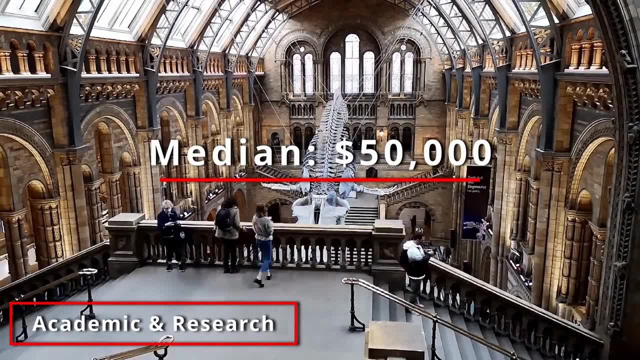 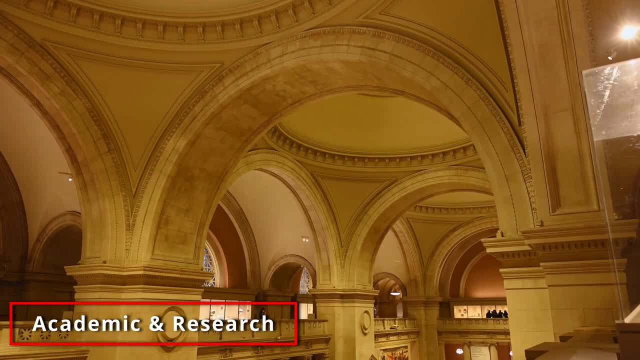 The median salary for people in these positions is about $50,000 per year. Getting a job as a museum curator often only requires a bachelor's degree as a minimum, but many organizations seek out experts in their field with many years of experience 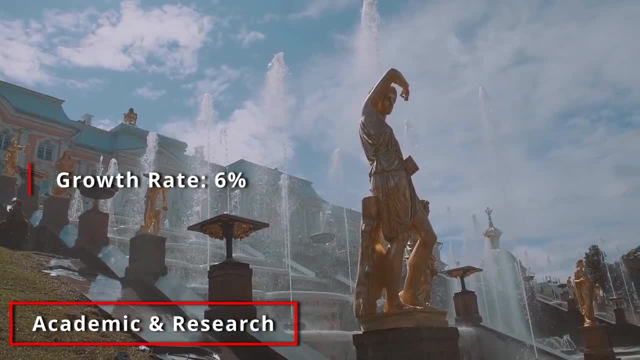 and at least a master's degree. This field is also on the rise, with a 6% predicted job growth rate over the next few years. 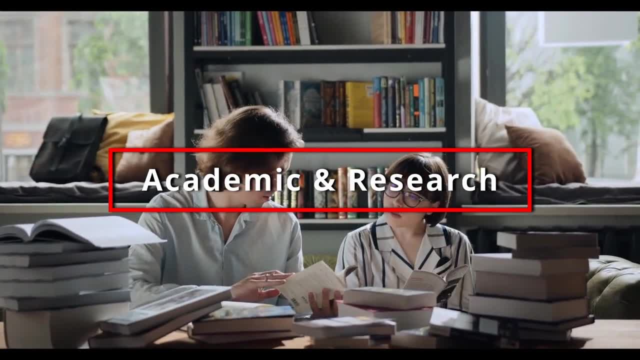 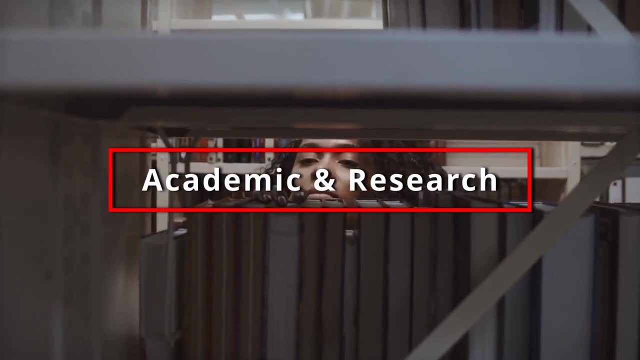 All of the different ways that academic research and education can take your job path can almost be mind-boggling. Fortunately, you can tailor your education to fit to what you want to do as a career. 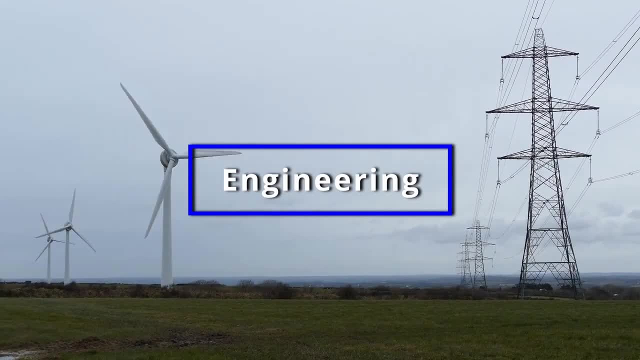 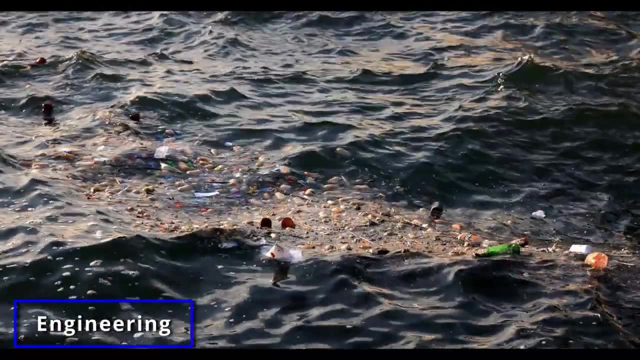 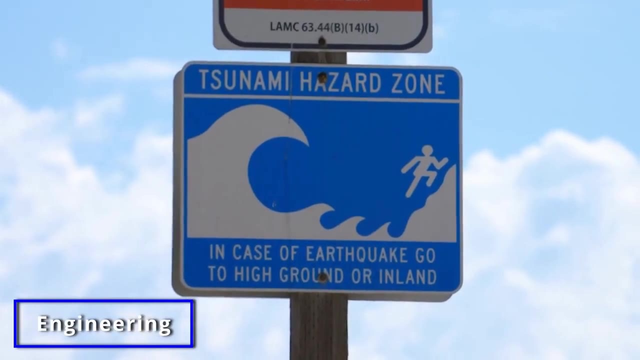 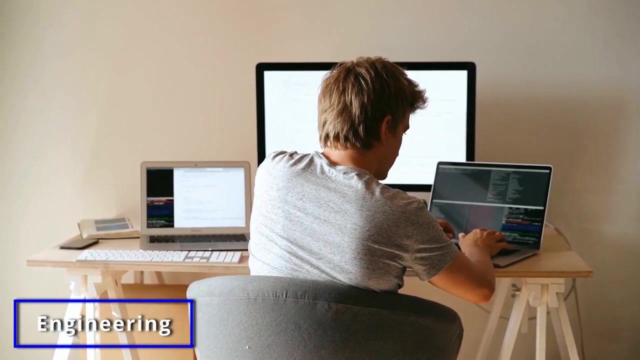 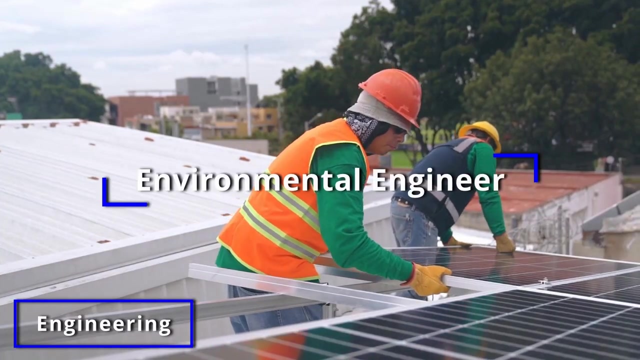 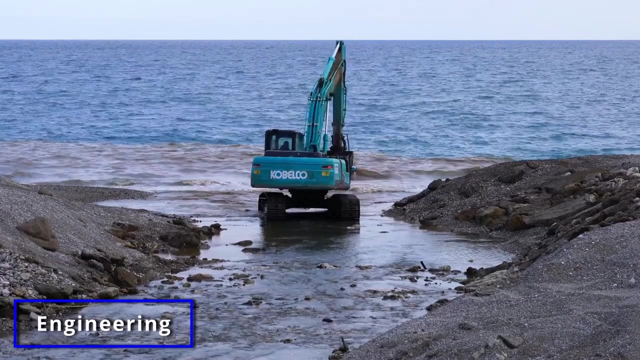 Engineering careers focus on the use of both environmental science and technology. Careers often involve developing better methods to understand infrastructure, pollution control, natural resources, public health, and other environmental problems in relation to humans. Anywhere from building infrastructure to better withstand earthquakes, to building water tanks, to developing new computer programs used in other sections of environmental sciences. These jobs often require perspective of other areas including atmospheric sciences, oceanography, hydrology, ecology, and biogeochemistry. Environmental engineers serve an important role in the engineering branch because they focus on how to integrate our technology with nature to both remediate and create a more sustainable way of life. 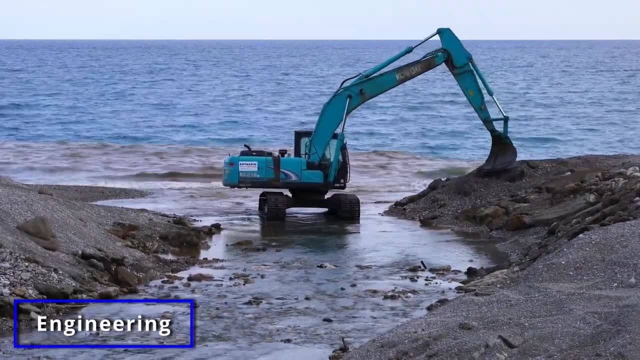 Like many jobs, people with this field in mind often specialize even further into areas like coastal management, ecology, and marine life. The field is often used to develop new computer programs for the use of other sections of environmental science and technology. 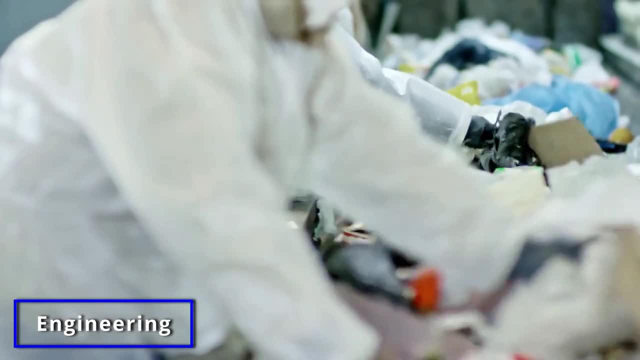 In a broad sense, environmental engineers work on projects to improve recycling, waste disposal, public health, and control of water, air, and land pollution. 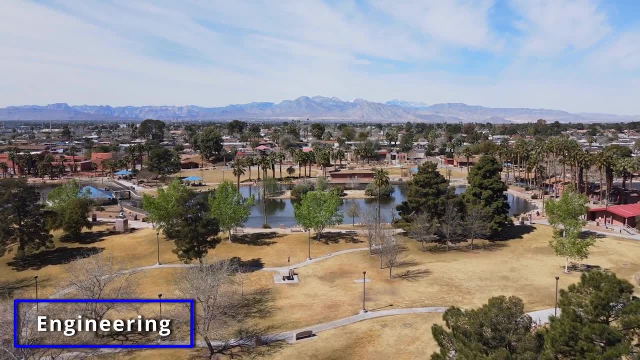 This job most strongly crosses with environmental and natural resource branches due to its focus on cleaning up and improving the sustainability of practices like mining and freshwater diversion. 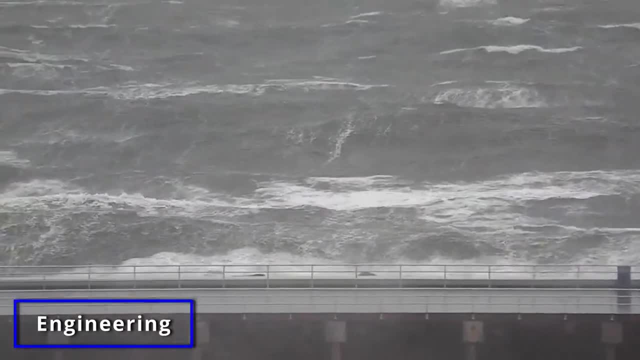 If you're looking to apply your engineering skills to your passion for keeping the planet healthy, this can be a great field to look into. An environmental engineer's median salary is around $67,000 per year. An environmental engineer's median salary is around $67,000 per year. An environmental engineer's median salary is around $67,000 per year. Most jobs require at least a bachelor's degree. 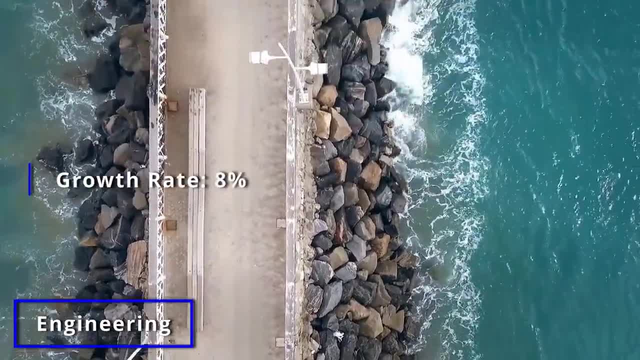 Most jobs require at least a bachelor's degree. This field is also very healthy, with an 8% predicted growth rate by 2030. 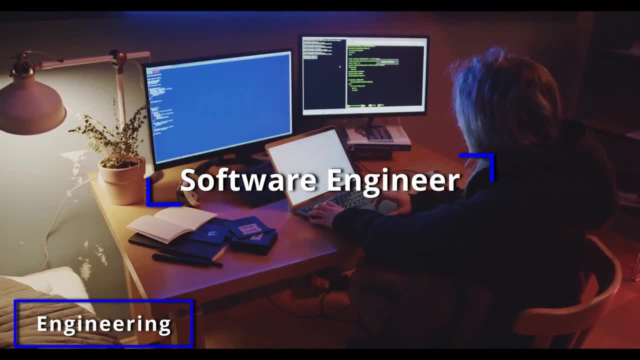 software engineering career duties involve designing computer programs, quality checks to identify any issues with these said programs, and working with other scientists to solve environmental problems. 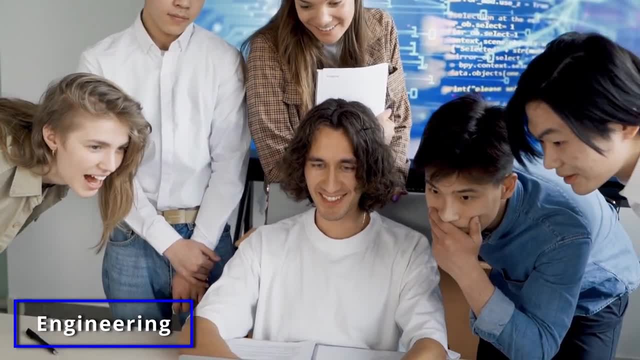 These robot programs assist Humans in their management of science and technology, and will also cut costs for others. 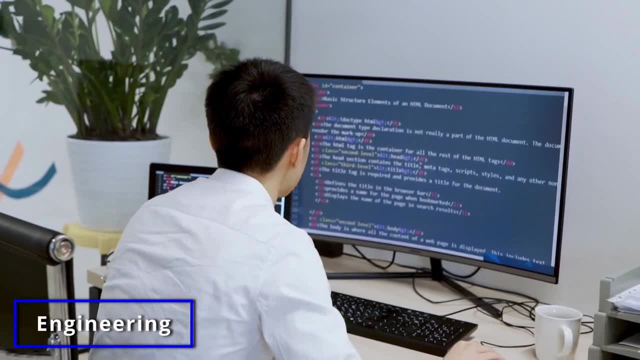 These careers are typically office jobs and most often require working on a team with other software engineers. 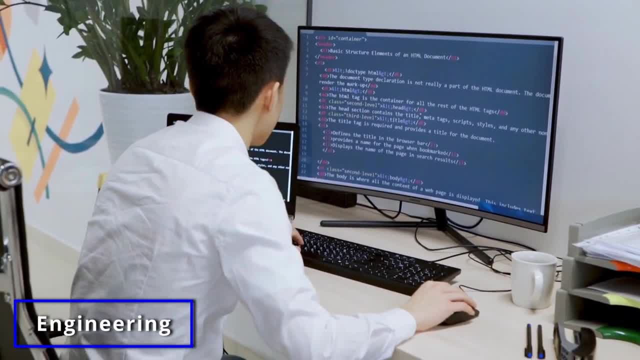 These jobs require a team withgemeister's are or sub-committee to optimize career development and 하 на� 효 ensuring that all Copper Nitrogen is regularly used. 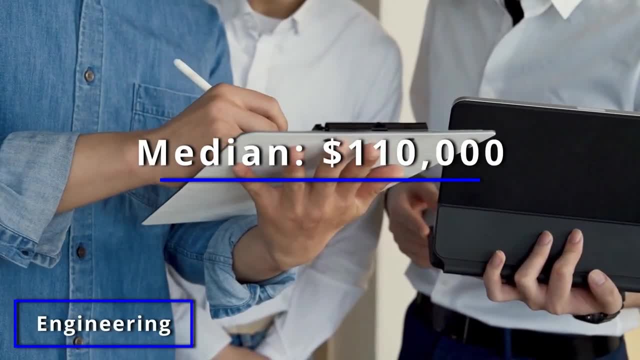 cereals are typically office jobs. and remote sensing fields. Median pay for software engineers is $110,000 per year. 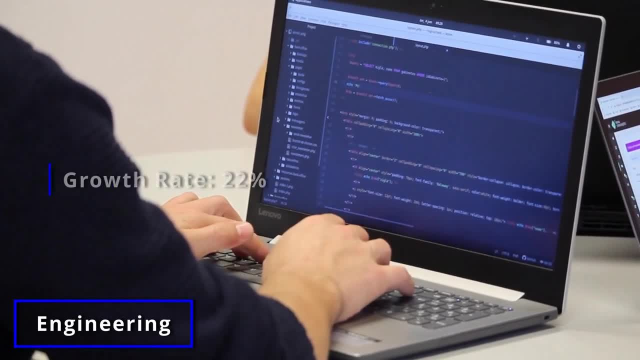 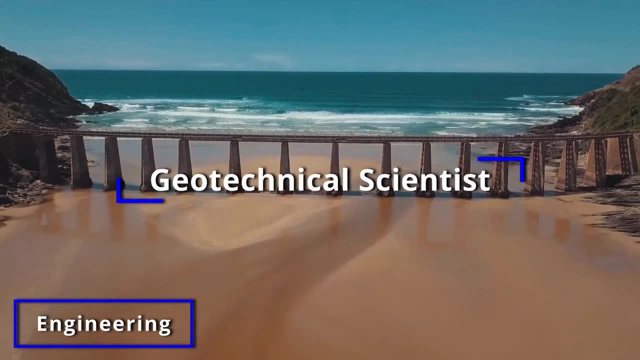 Typical entry-level jobs require a bachelor's degree, and careers in this field are projected to grow 22% by 2030, which is above average. Geotechnical scientists research and study soil to evaluate its suitability for foundations. They investigate and assess construction sites, 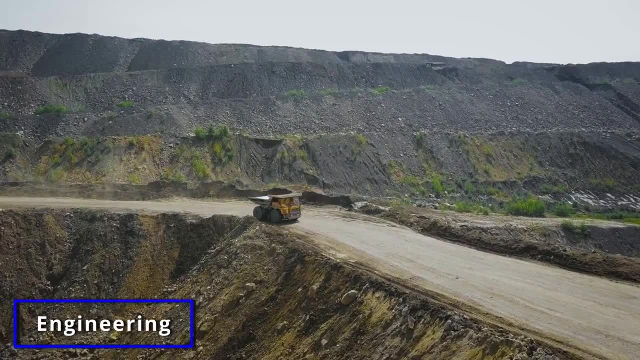 conduct lab tests, create designs for structures, supervise construction, write and present reports. 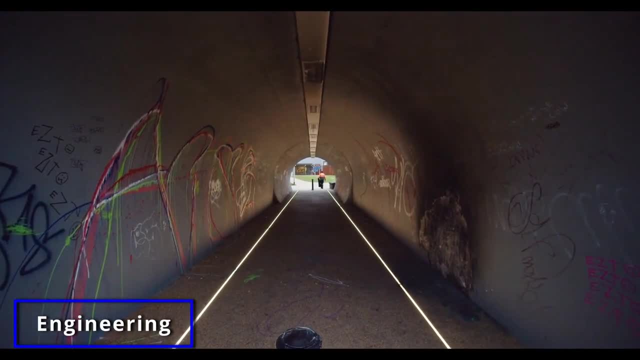 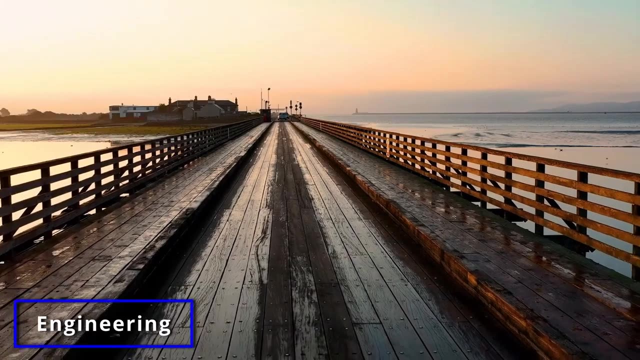 They work on projects such as designing tunnels, roadways, retaining walls, and earthen dams, as well as help to create strategies for the cleanup and management of contaminated sites. 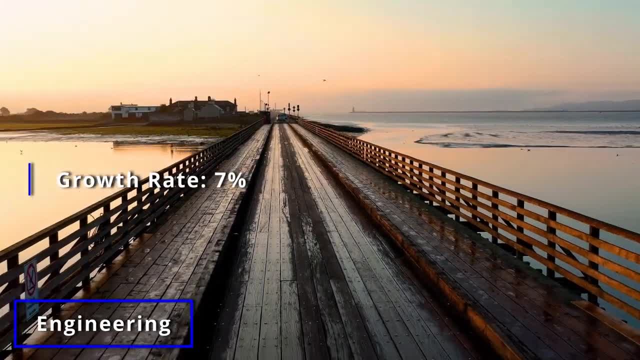 This field has experienced a job growth of 7%, and the mean pay of these jobs is $75,000. 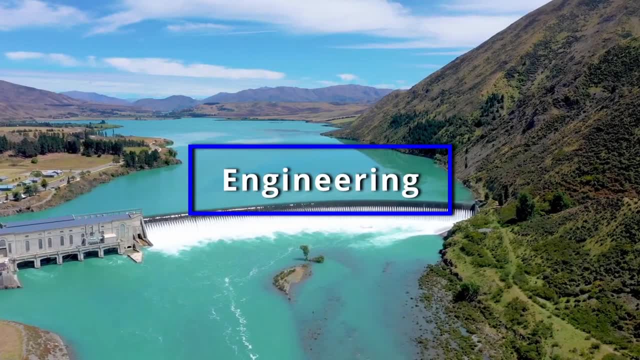 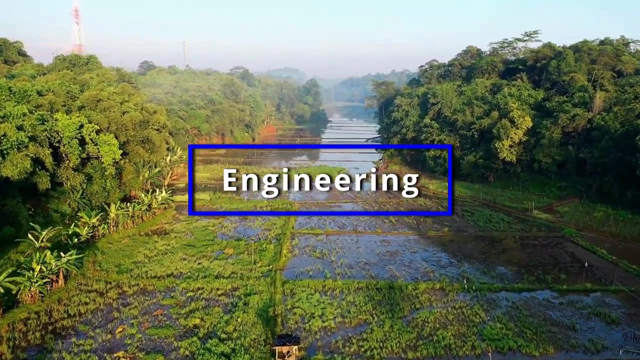 Careers in engineering most often have overlap with the environmental and remote sensing fields, but may have overlap in others. The engineering field is diverse and a great option for those who enjoy teamwork and problem solving. 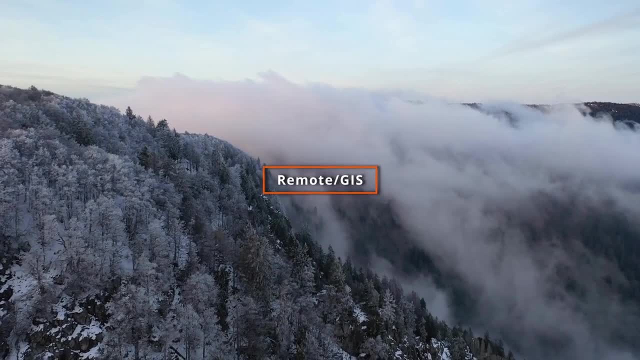 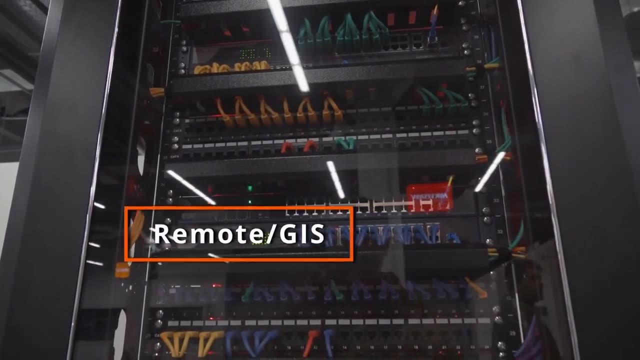 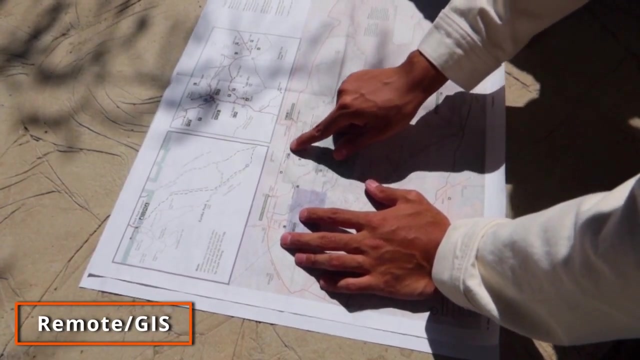 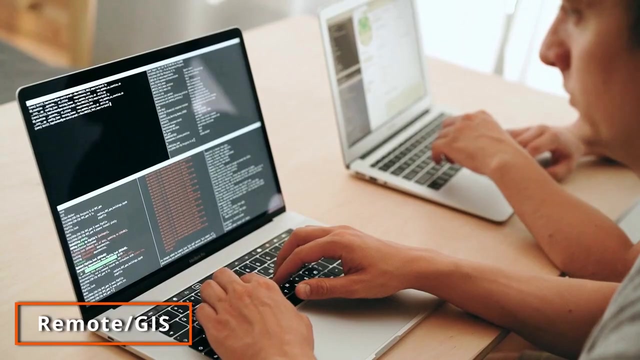 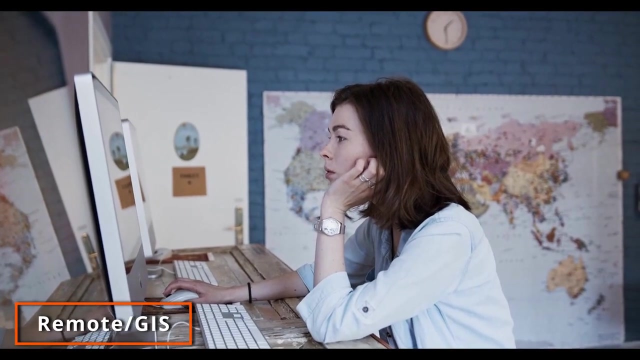 Remote sensing and GIS work has become a vital part of our everyday world, and continues to become more so with the constant evolution of computer technology to boast it. Massive datasets can be analyzed in a fraction of the time, more detailed geographical and geological maps can be auto-generated with proper programming, and thousands of miles of terrain can be viewed in a day to find the perfect site conditions. Knowledge of commonly used code bases like Python and R, as well as the ability to navigate GIS software like ArcGIS Pro will quickly set you in the running as a competitive candidate for many of these available jobs. 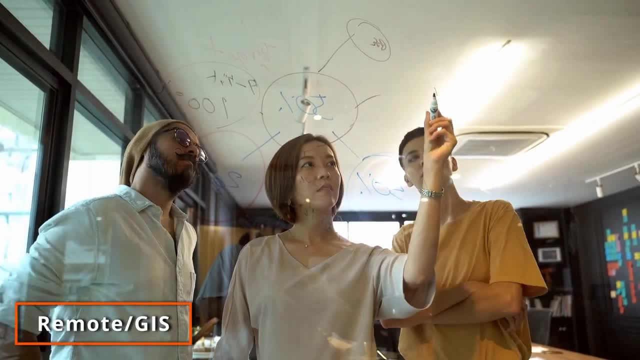 Some common knowledge sets people in this field bring to the table include mathematics, statistics, computer science, and physical geography. Capable people in this field are invaluable to modern projects of all kinds. 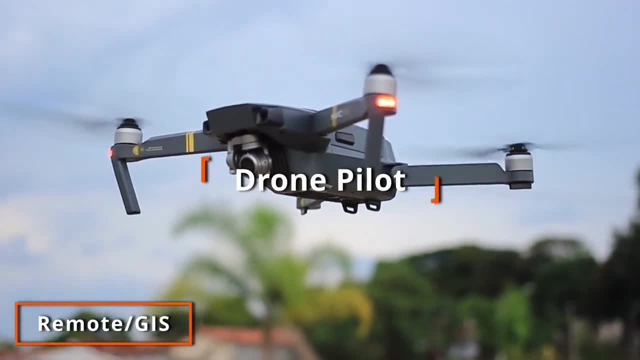 A new career path that is really taking off is being a drone pilot. Drones excel at taking over jobs that are dark, dirty, and dangerous, like mapping underground sewage and electricity 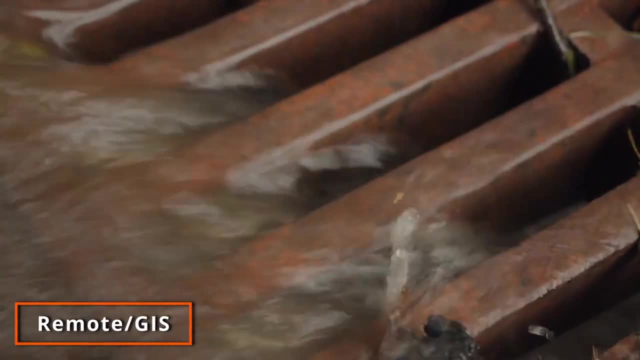 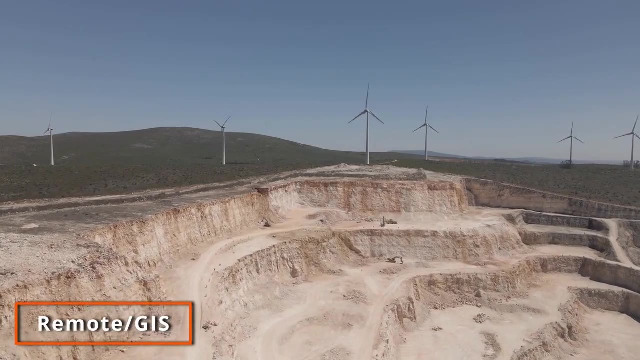 tunnels for a city. There are many other uses for drone technology like identifying subsurface conditions for construction companies, oil and gas pipelines, and strip mining conditions. 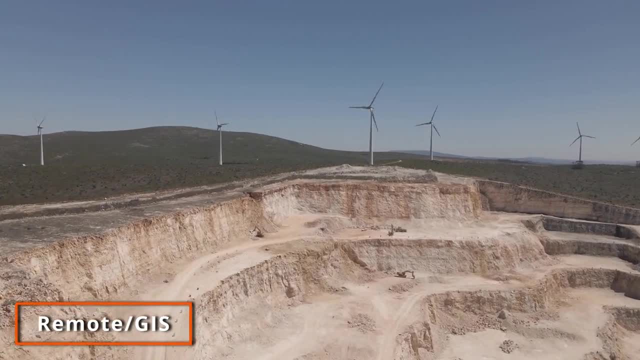 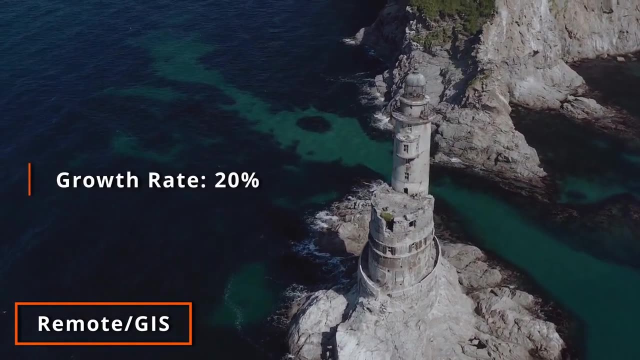 While there are no college paths to becoming a drone pilot, there are certification training and testing programs all over the country. We even pay $60,000 per year, with a 20% compounded yearly growth rate until 2031. This data was culled and averaged from several job and career 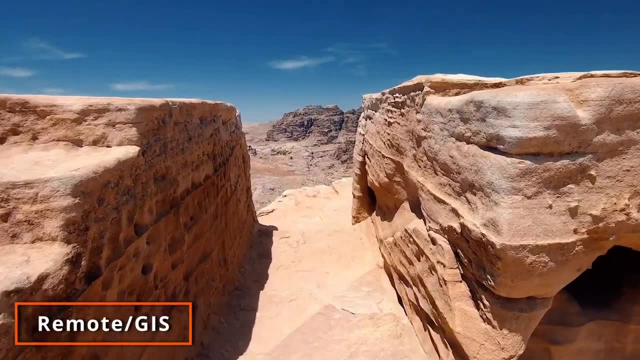 websites as the profession is still young enough that the Bureau of Labor Statistics has not published any statistics on this career. 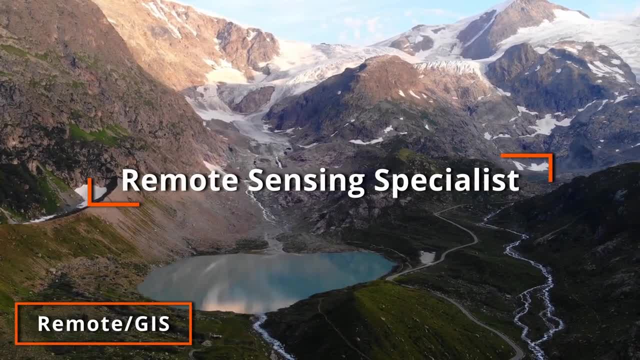 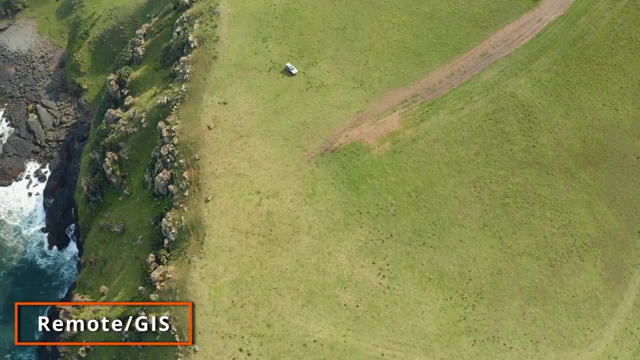 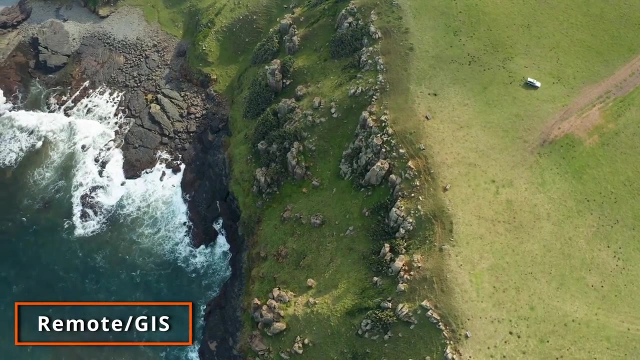 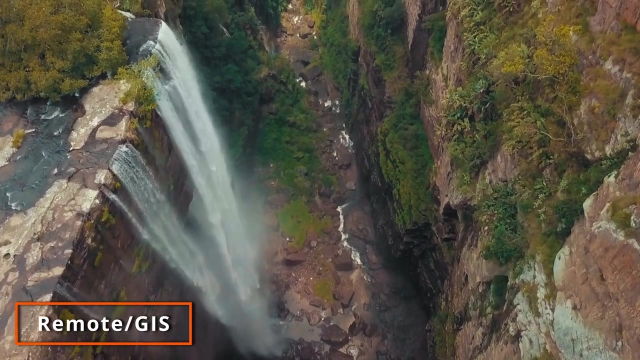 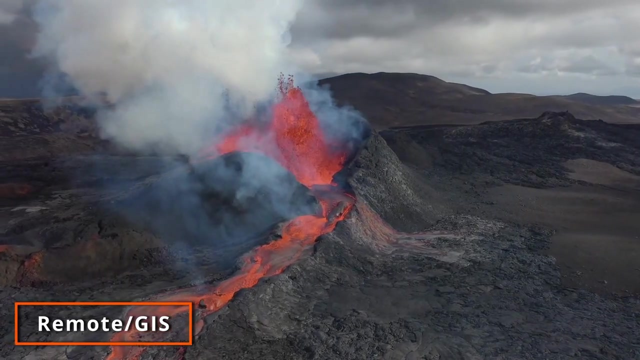 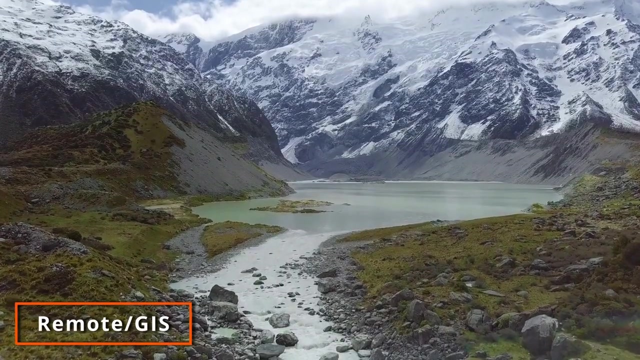 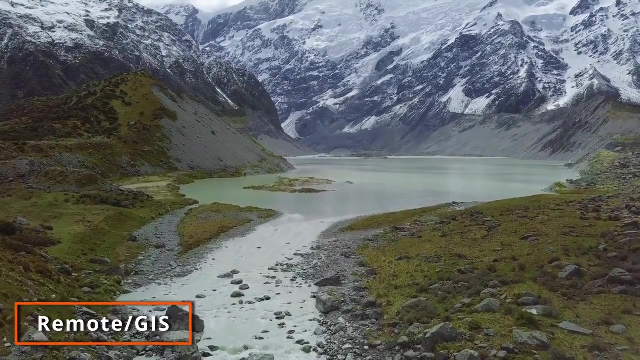 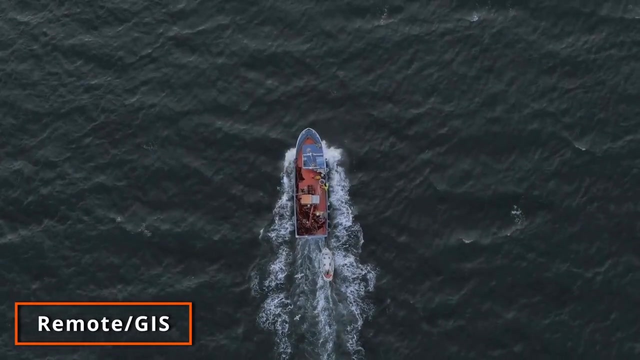 Remote sensing specialists serve as an important part of many large-scale operations due to their ability to view and analyze massive areas all over the world. This job can have many phases and expectations, but some common practices consist of the analysis of aerial and satellite imagery along with LIDAR and sonar data to determine ground composition, characteristics, and cover. As for the sites themselves, they vary greatly, but can include those that are difficult or impossible to access, some even dangerous. One important aspect is that some of the data can be used for risk assessment of a project site against local obstacles and natural disasters. Remote sensing applications are not specific to any one sector, but rather can be helpful in one way or another to them all. While it's necessary to have boots on the ground for in-person observation, it's equally valuable to have people who can view the larger picture. Between the money invested in these projects and the scale of them, people with this job are often well-paid, with an average salary over $80,000 per year. 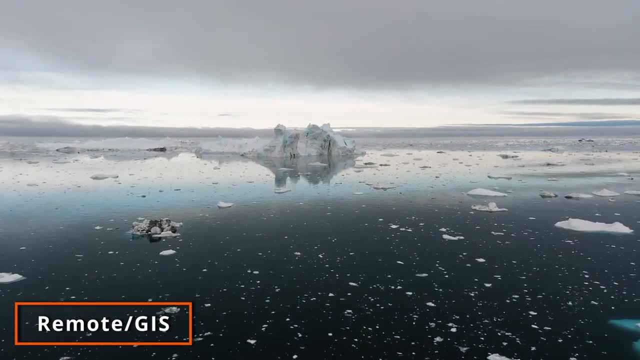 For education, most professionals do not have to pay $100,000 per year to get a job. For education, most professionals do not have to pay $100,000 per year to get a job. For education, most professionals do not have to pay $100,000 per year to get a job. For education, most professionals in these positions have a bachelor's degree or higher. Although slightly lower than some 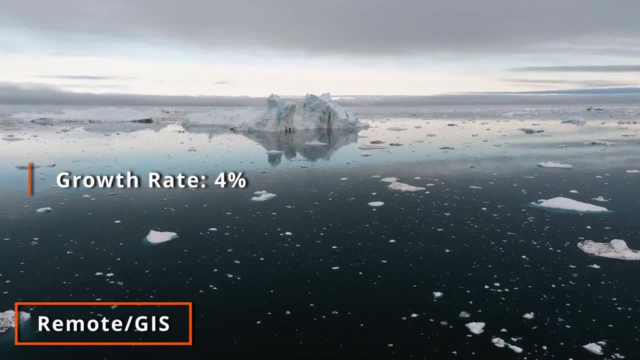 others on our list, this field is still growing, with an expectation of around 4% by the year 2030. 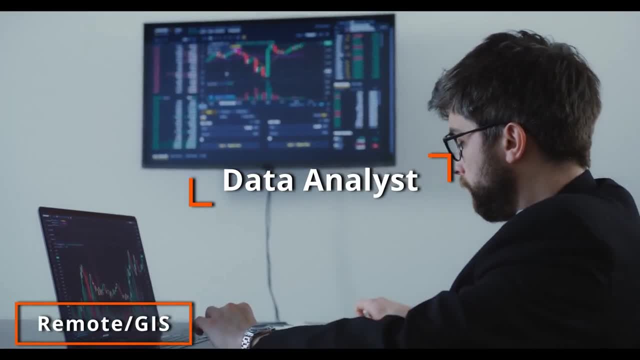 Environmental data analysts tend to focus in statistics, working with market research, environmental data, and other business information to make it accessible to the general public. 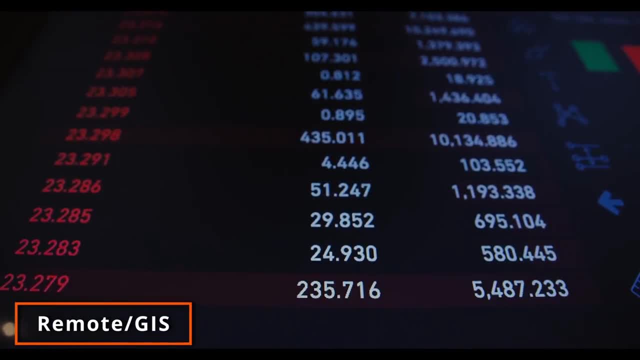 Environmental data can include climate, contaminants, natural hazards, and more. Students who enjoy working with numbers and technology will find careers in this field appealing. Typically, these scientists work in the field of environmental data analysis, which includes environmental data analysis, which includes environmental data analysis, and other business-related studies. 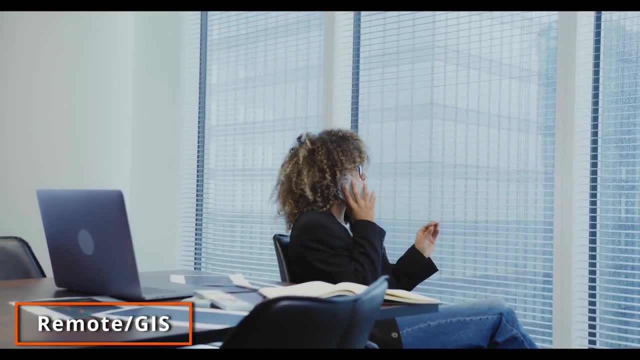 Most scientists work in mostly office settings, with travel being necessary depending on the client. There is overlap with the environmental, natural resources, and engineering fields. 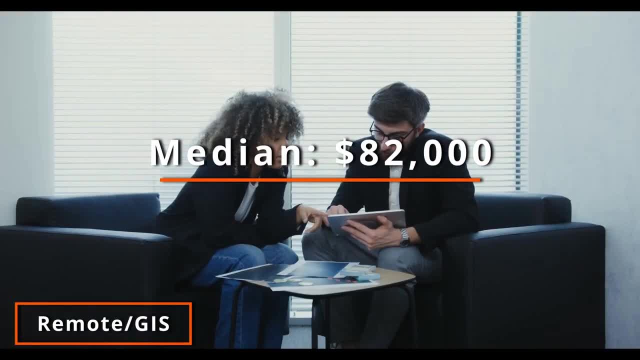 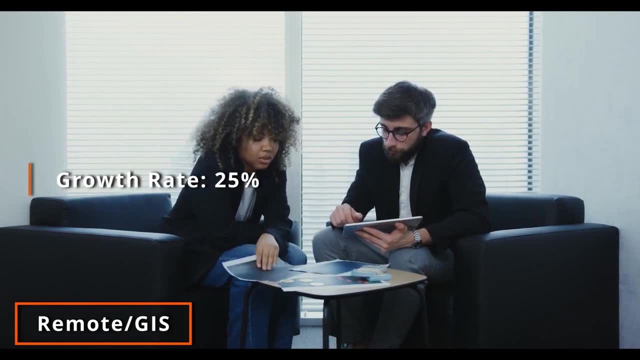 Median pay for data analysts is $82,000 per year. Typical entry-level jobs require a bachelor's degree, and careers in this field are projected to grow 25% by 2030, which is above average. 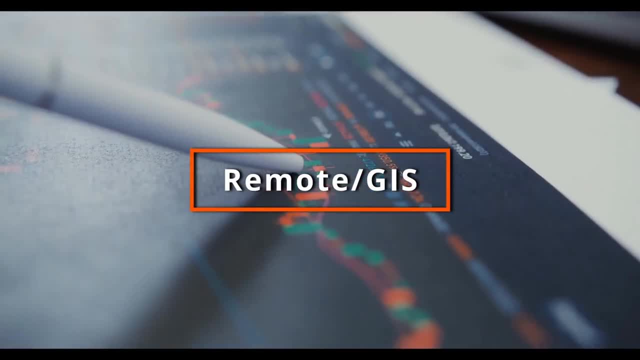 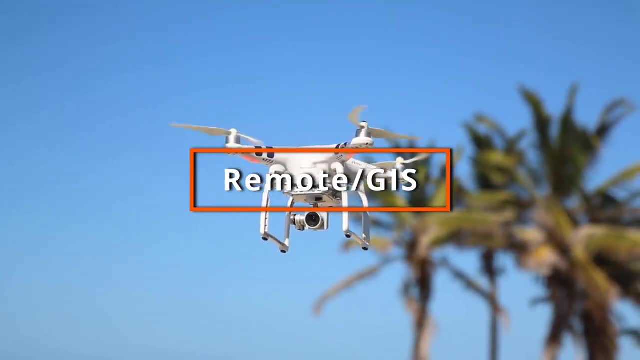 If you enjoy combing over massive data sets, operating UAVs, designing maps, or writing code, then this branch should be high on your list. The growth for these jobs is often higher than average, and so is the pay, all while providing a comfortable office job at least some of the time.